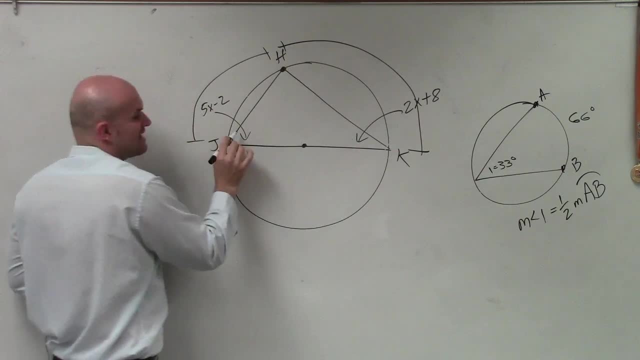 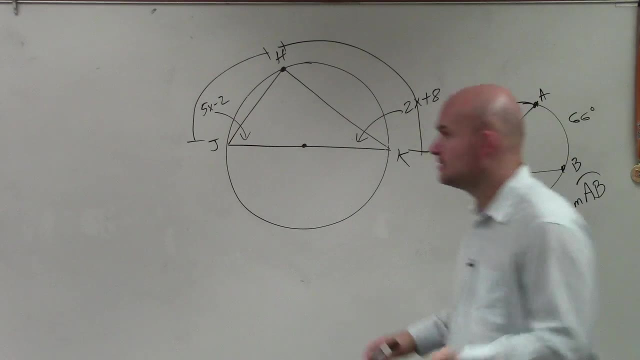 OK, And this angle is 1 half that arc. Again, we don't know the measurements of the arcs, but we know that it's going to be 1 half of that. Now, what we do know is this creates a semicircle, correct? 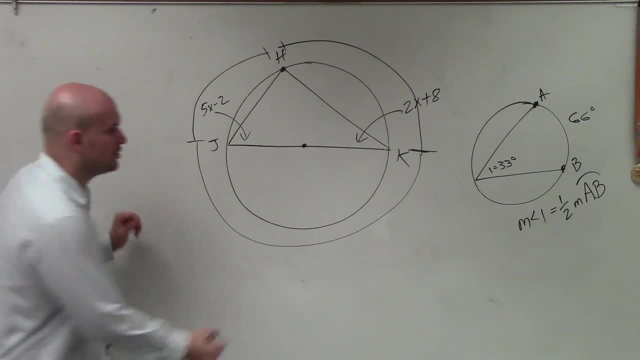 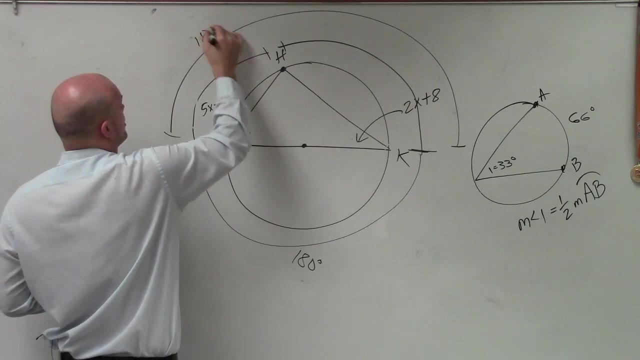 And the semicircle is 180 degrees, So the measure of the arc is 180 degrees. So what that means is the measure of this arc is also 180 degrees, right, Because that's another semicircle. So when we're trying to construct an equation, 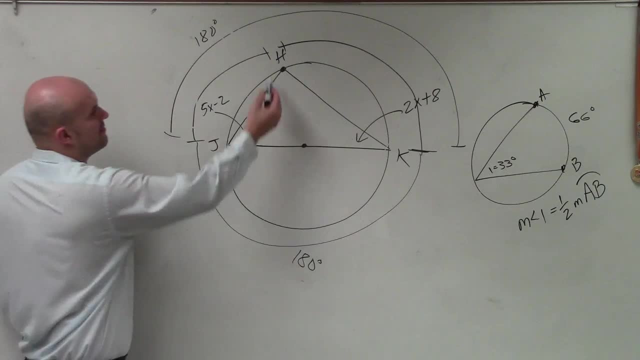 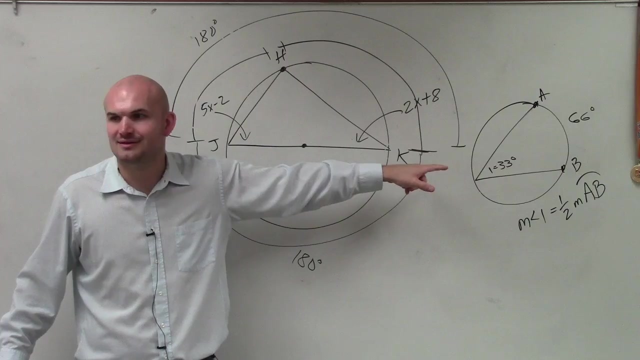 to solve for our missing variables. what we notice is the measurement of these two arcs add up to Jake. what do these two arcs add up to, This arc plus that arc? I don't know why I want to keep on calling you Jake. 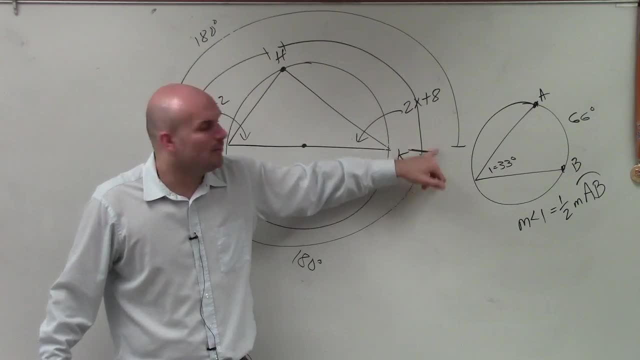 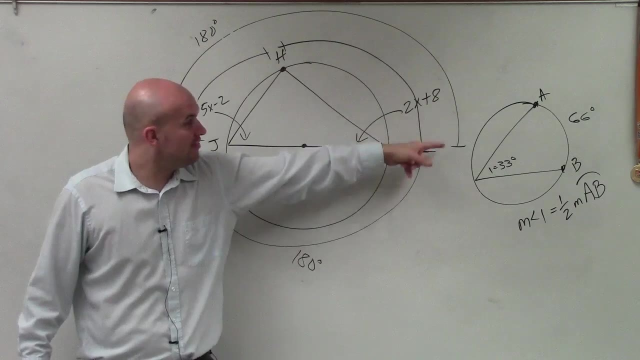 Maybe that's it. So I guess, Jake, I'll ask you the question then: What do these two arcs add up to? OK, well, the number is: since this arc adds up to 180,, this whole arc adds up to 180. 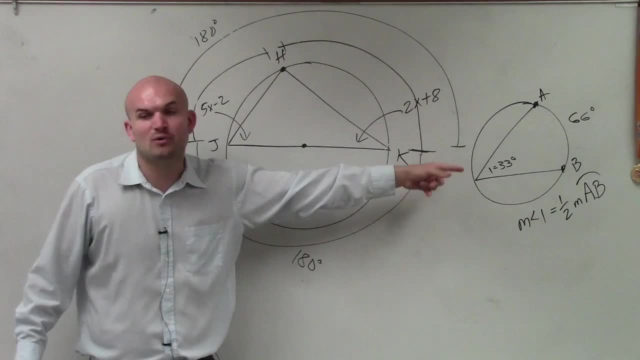 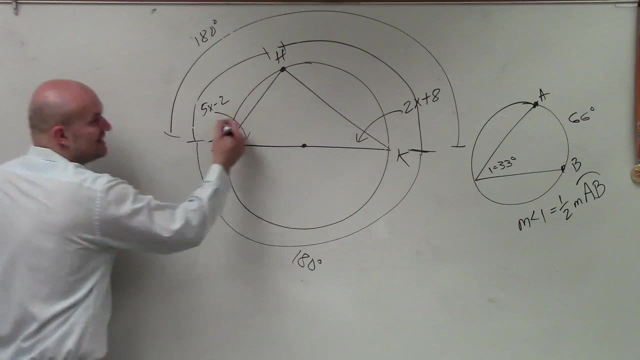 So what I'm simply asking is, when you break up these two arcs into 180, then you can say that the sum of these two is to 180.. So therefore, these two add up to 180, but we're not remember the arc's inscribed angle. it's 1 half of that. 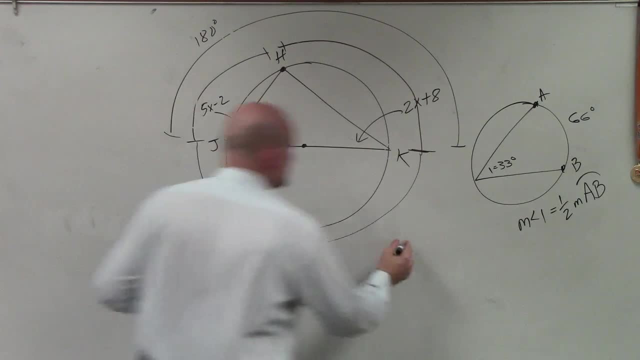 So these two add up to 1 half of 180, which is 90. So the equation I'm going to write, which I'll write over here, is 5x minus 2.. OK, OK, OK, OK, OK. 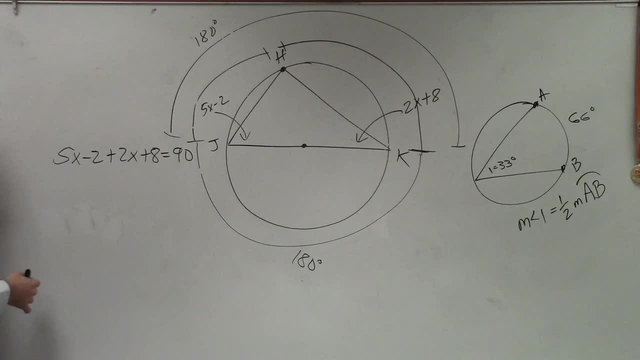 So what I'm going to write is: 2x plus 8 equals 90 degrees. They don't add up to 180.. They add up to 90. Because if they were central angles, they would add up to 180.. Since they're not central angles, 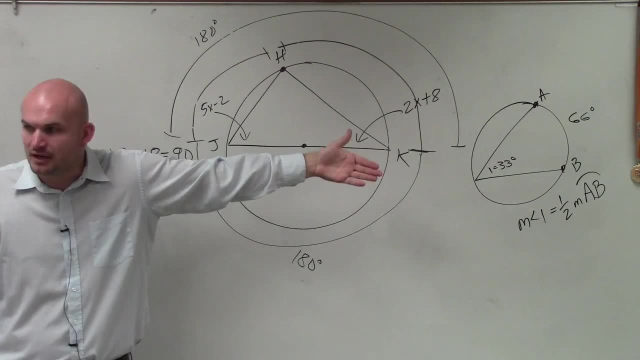 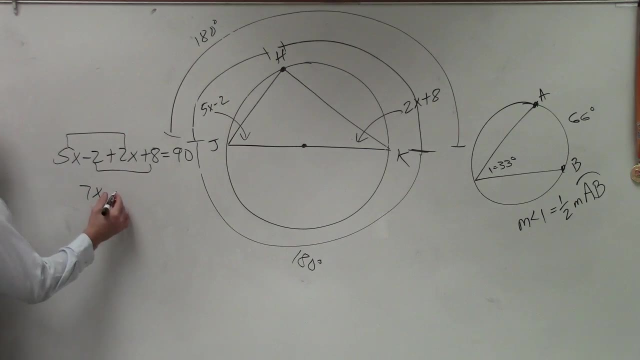 they're inscribed angles. they add up to 1 half of our arc measure, So that's 90. Now I combine my like terms and I get: 7x plus 6 equals 90.. Sorry, Robert, I don't really want to have to do this for the whole class.